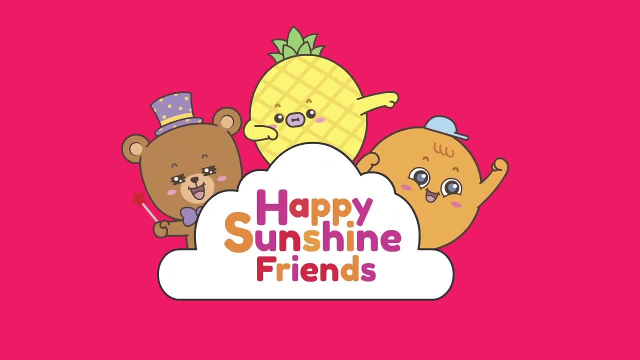 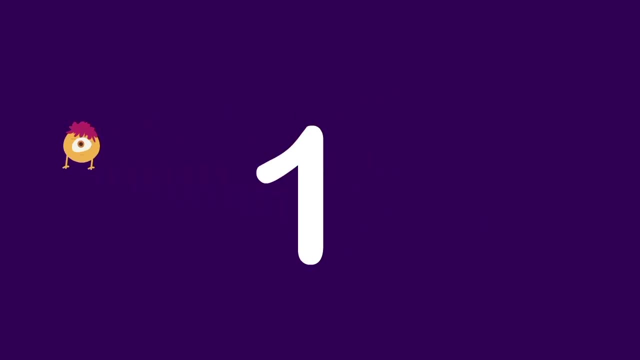 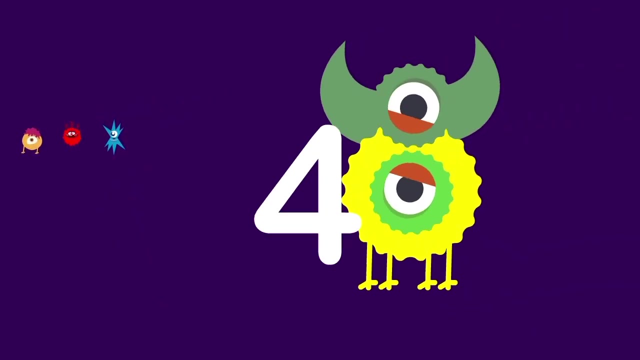 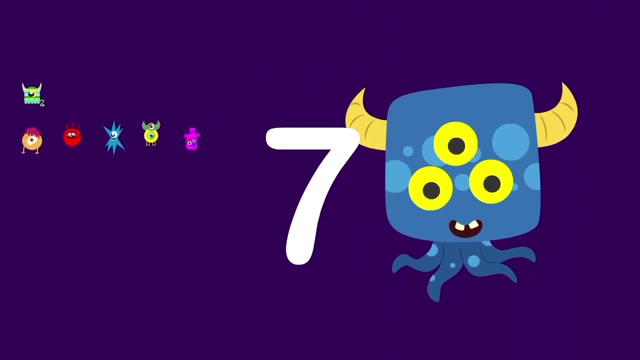 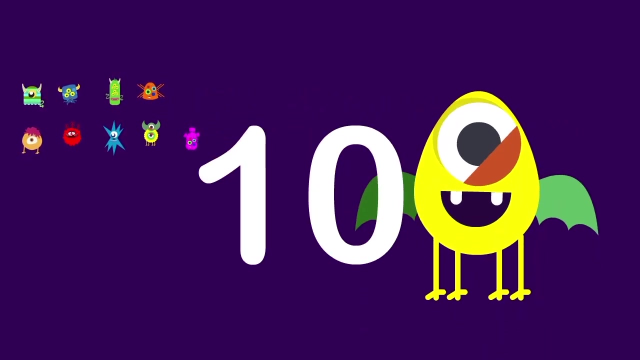 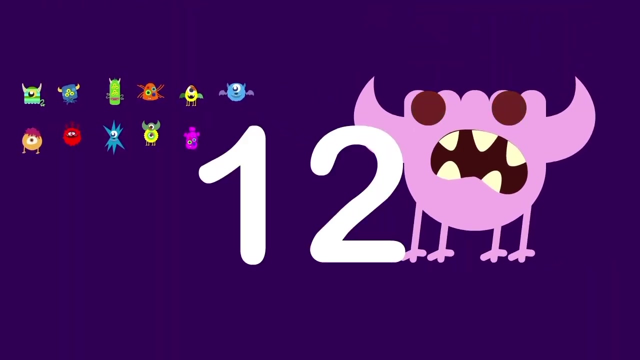 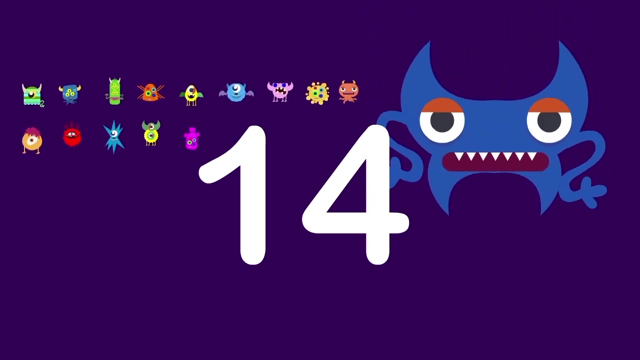 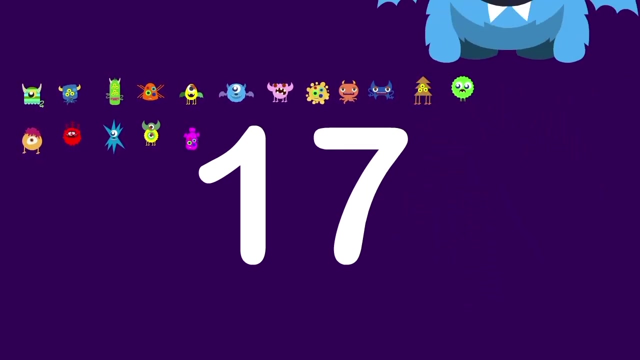 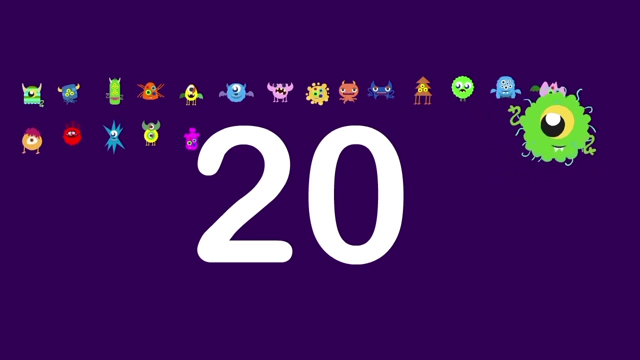 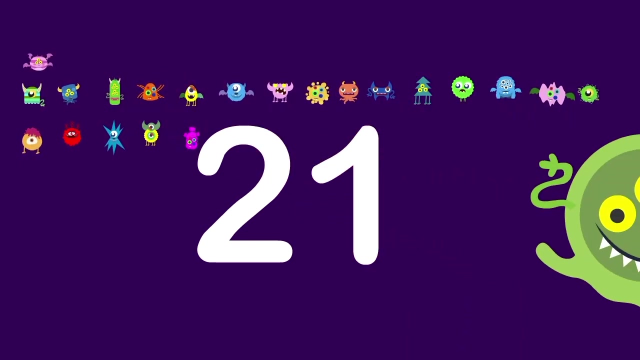 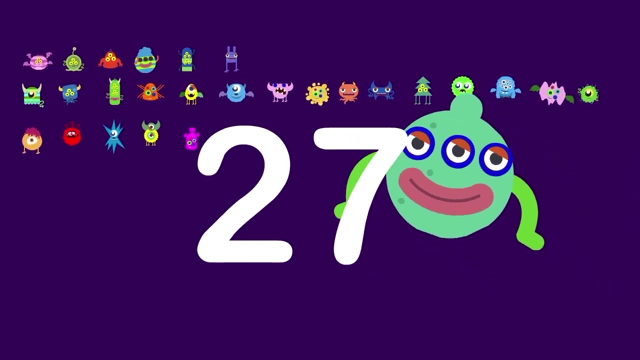 Happy Sunshine Friends. 10,, 10,, 11,, 12,, 13,, 14,, 15,, 16,, 17,, 18,, 19,, 20.. 20,, 21,, 22,, 23,, 24,, 25,, 26,, 27,, 28,, 29,, 30. 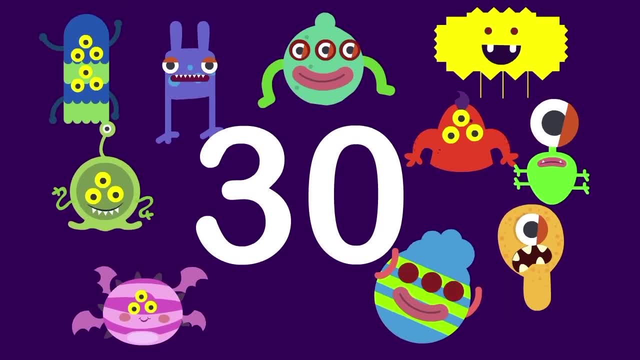 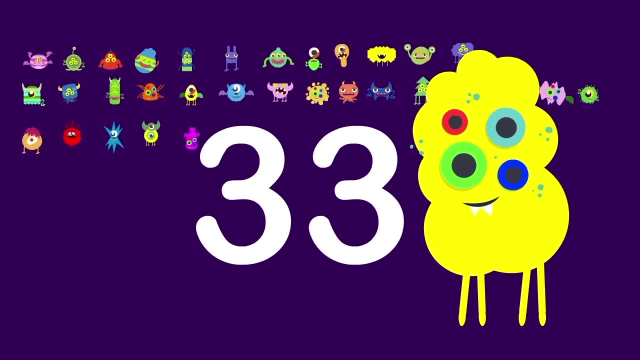 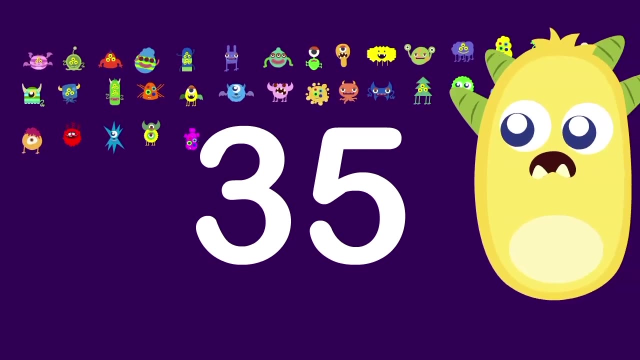 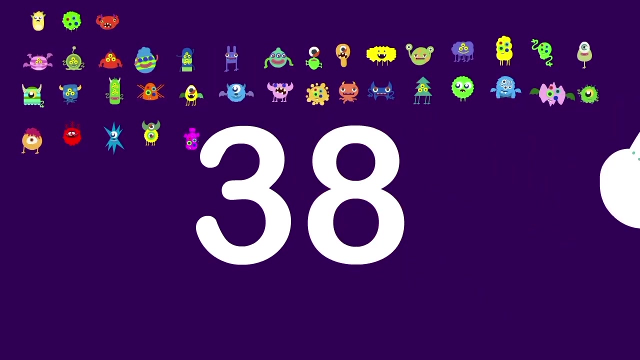 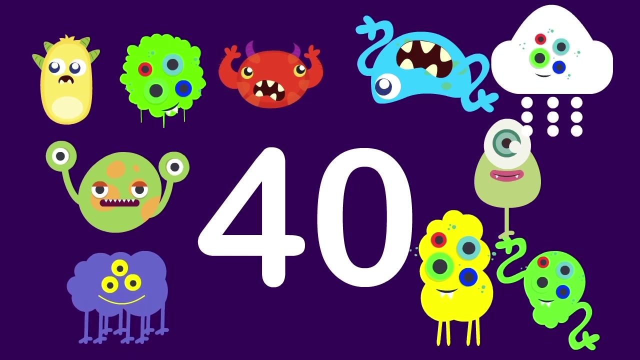 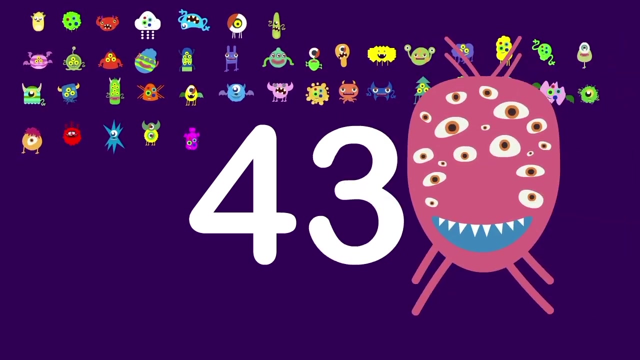 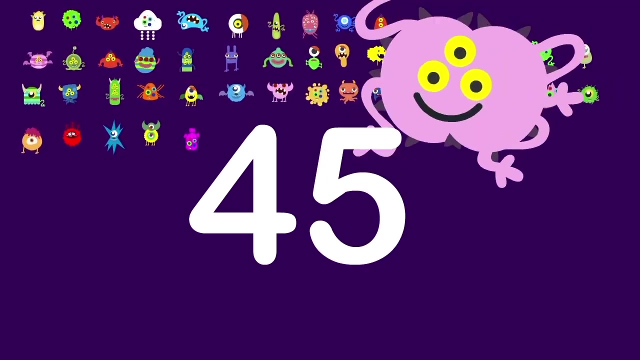 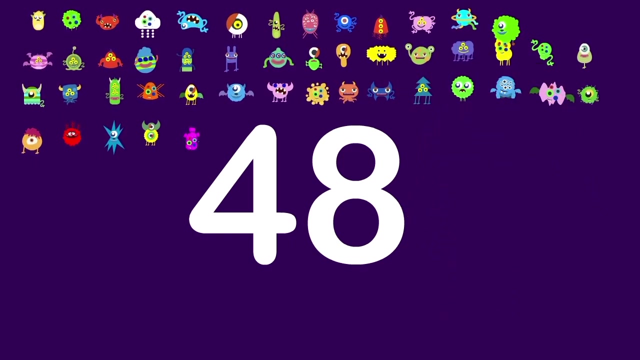 30.. 30.. 30,, 31,, 32,, 33,, 34,, 35,, 36,, 37,, 38,, 39,, 40.. 40., 40., 41,, 42,, 43,, 44,, 45,, 46,, 47,, 48,, 49,, 50. 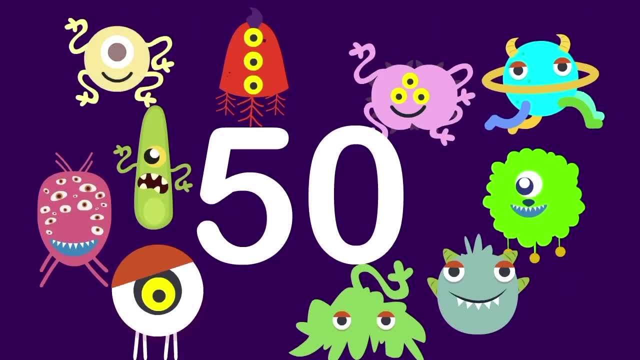 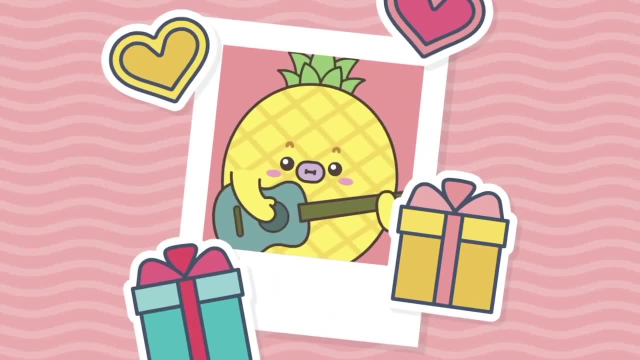 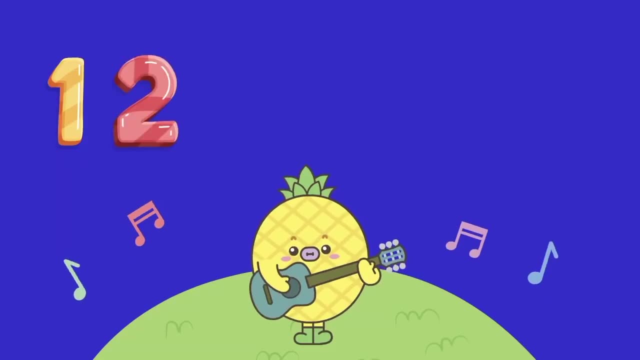 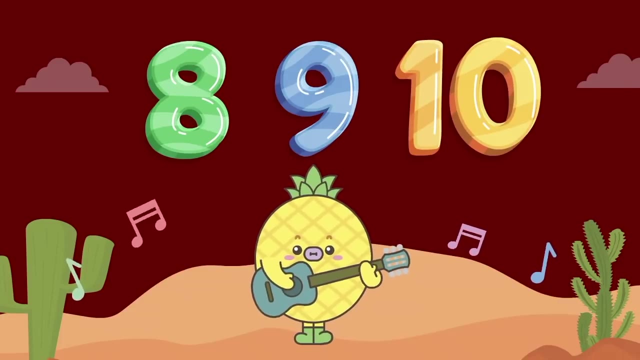 50.. 50.. 50.. 50.. 1,, 2,, 3,, 4,, 5,, 6,, 7,, 8,, 9,, 10,, 8,, 9,, 10.. 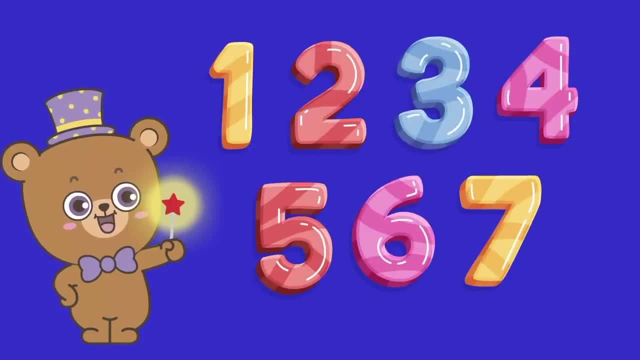 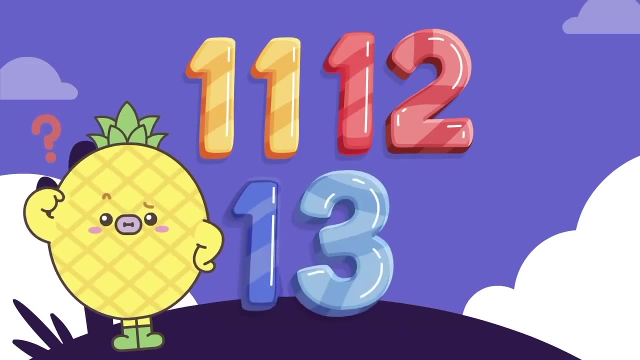 1,, 2,, 3,, 4,, 5,, 6,, 7,, 8,, 9,, 10,, 8,, 9,, 10. 11., 12., 7. 7.. 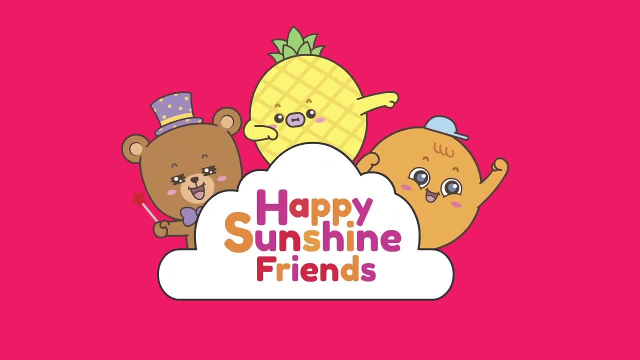 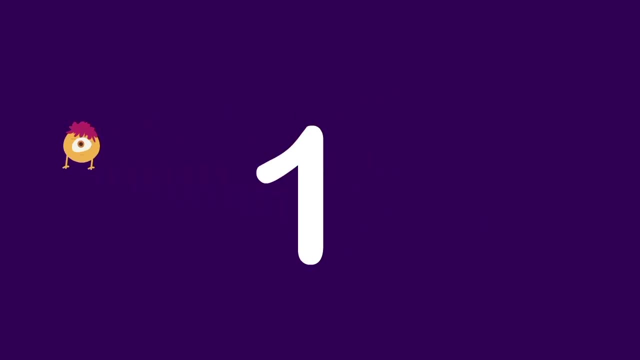 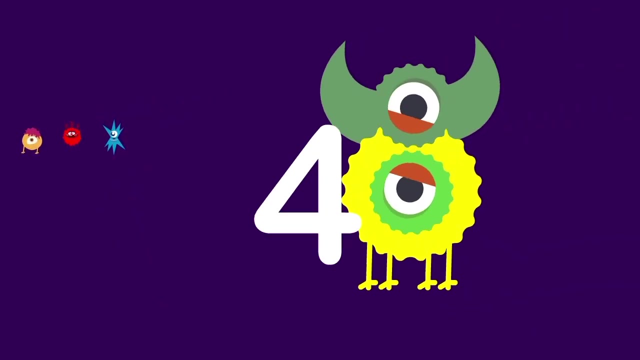 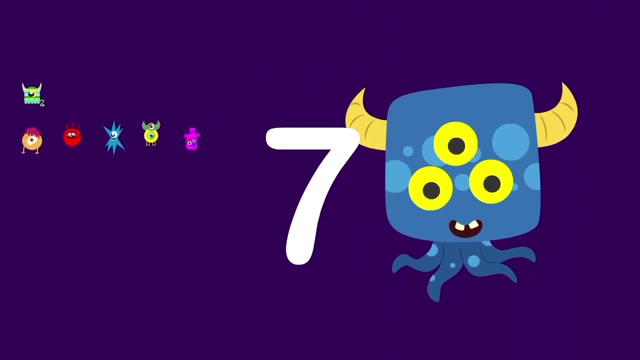 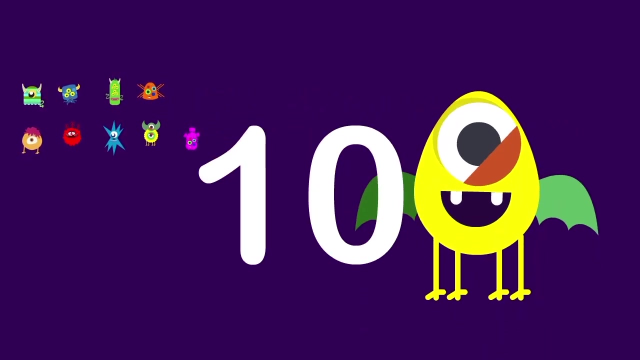 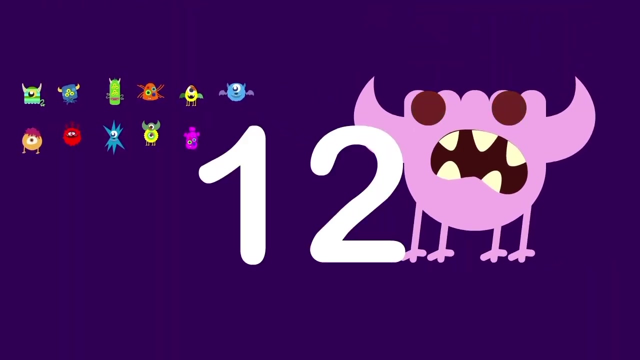 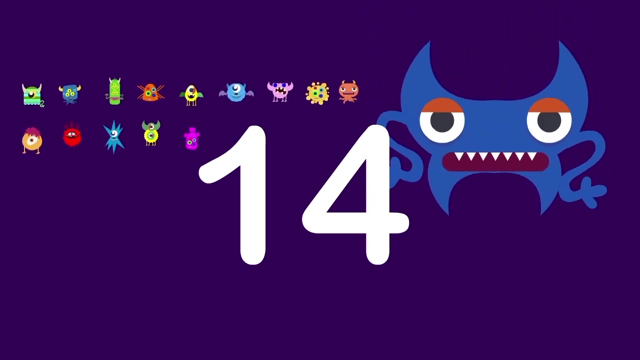 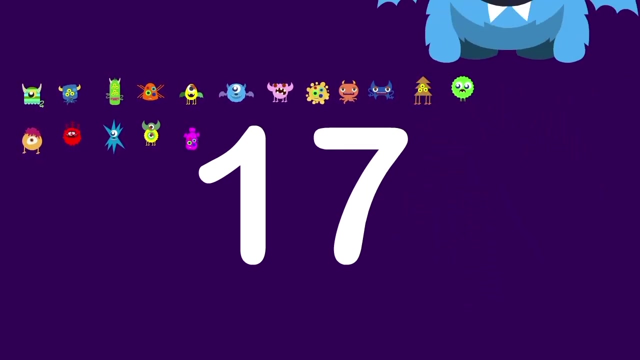 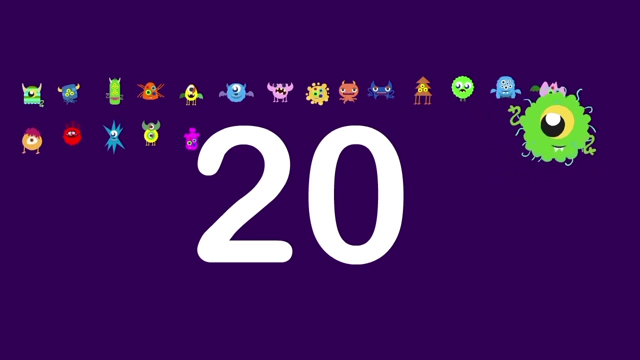 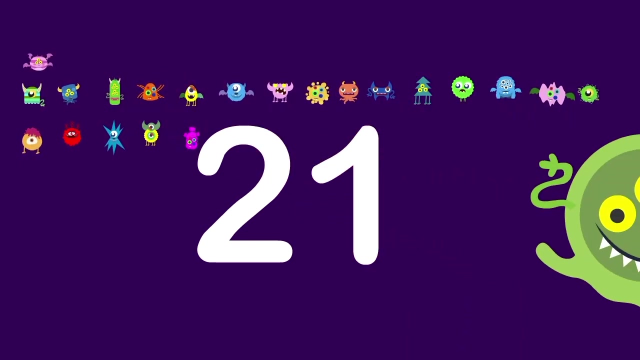 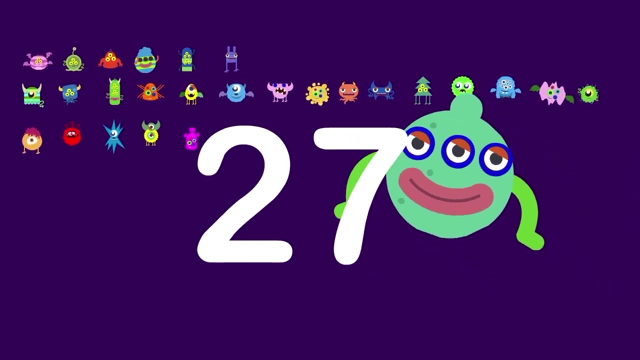 Happy Sunshine Friends. 10,, 10,, 11,, 12,, 13,, 14,, 15,, 16,, 17,, 18,, 19,, 20.. 20,, 21,, 22,, 23,, 24,, 25,, 26,, 27,, 28,, 29,, 30. 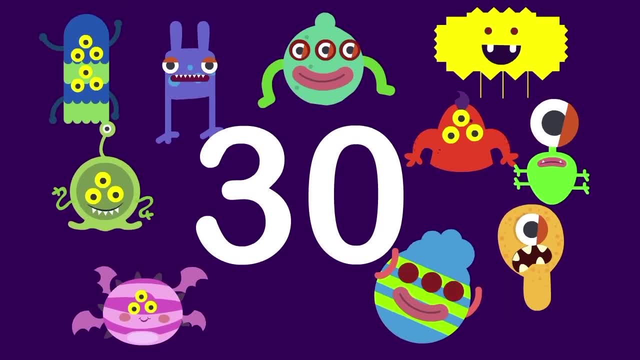 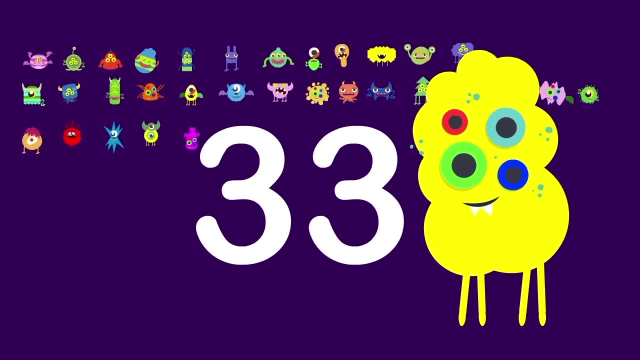 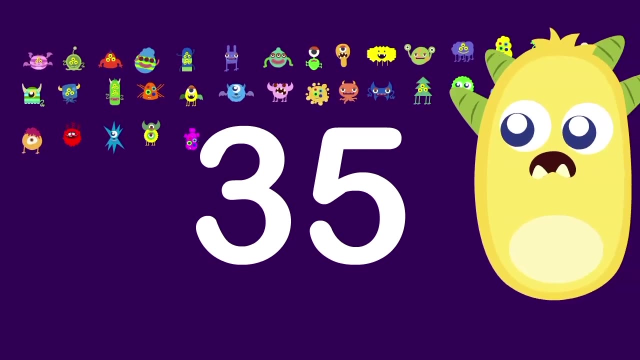 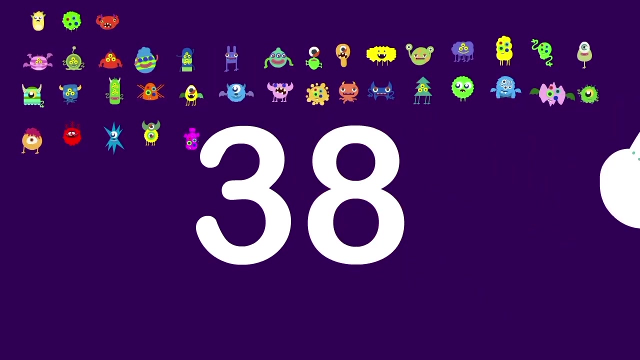 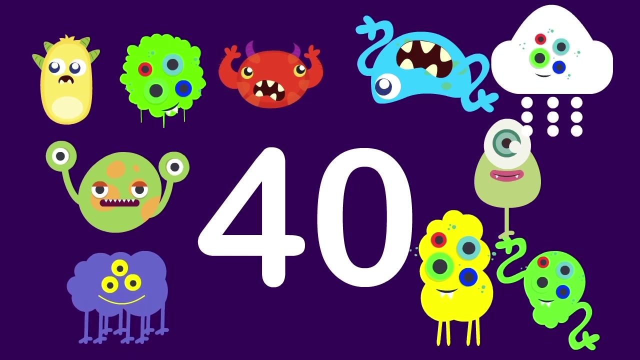 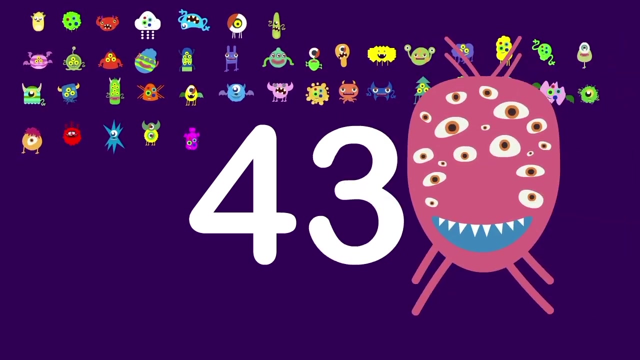 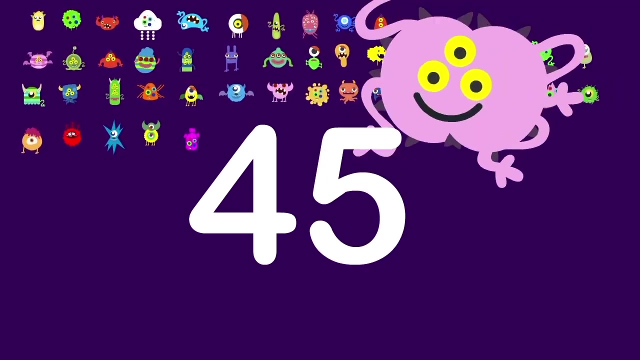 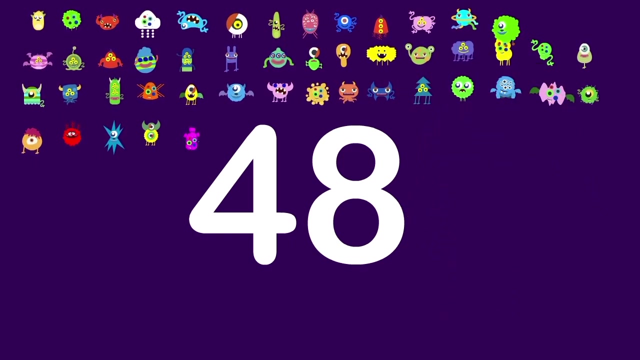 30.. 30.. 30,, 31,, 32,, 33,, 34,, 35,, 36,, 37,, 38,, 39,, 40.. 40., 40., 41,, 42,, 43,, 44,, 45,, 46,, 47,, 48,, 49,, 50. 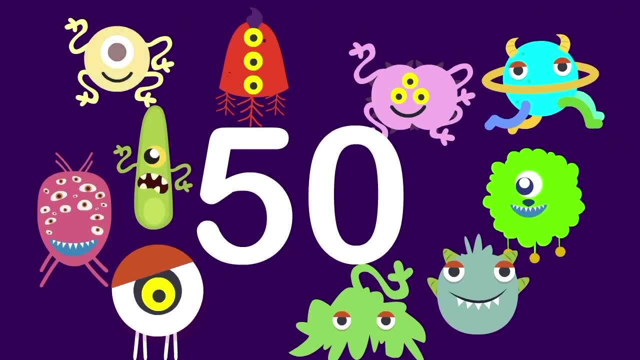 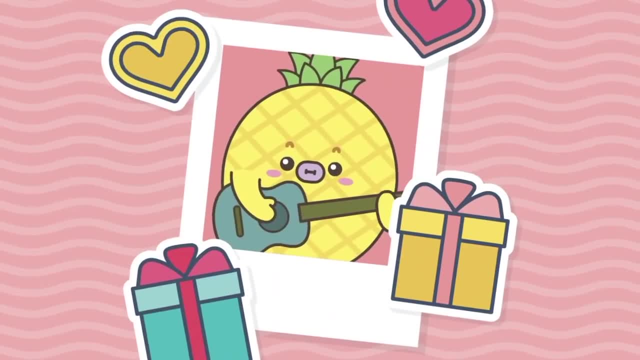 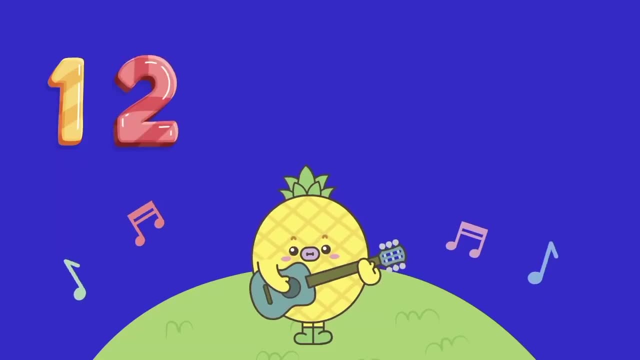 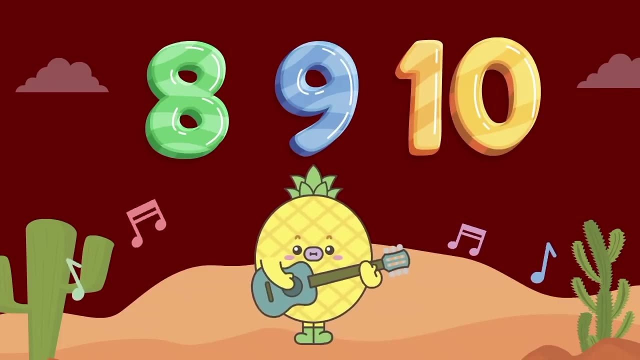 50.. 41,, 42,, 43,, 45,, 46,, 47,, 49,, 50., 70., 70.. 1,, 2,, 3,, 4,, 5,, 6,, 7,, 8,, 9,, 10,, 8,, 9,, 10..